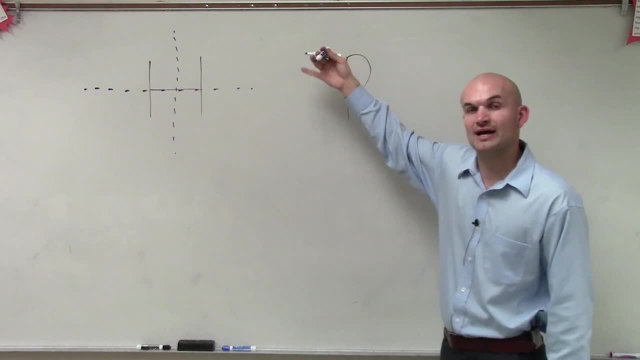 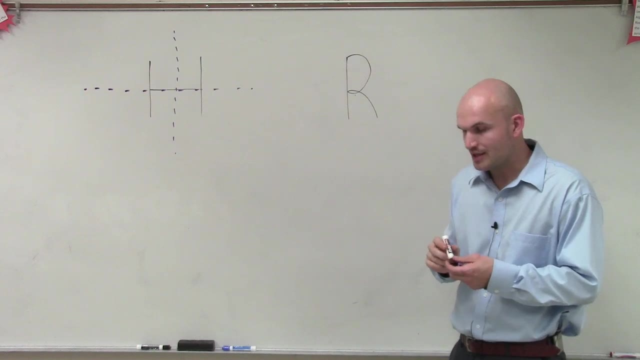 of symmetry. There's no way I can draw a line where one part of the letter is going to be exactly a duplicate of the other part of the letter. So remember, that's just a quick little overview of lines of symmetry. Now let's go and take a look at a parabola and see what is going to be the line of symmetry. 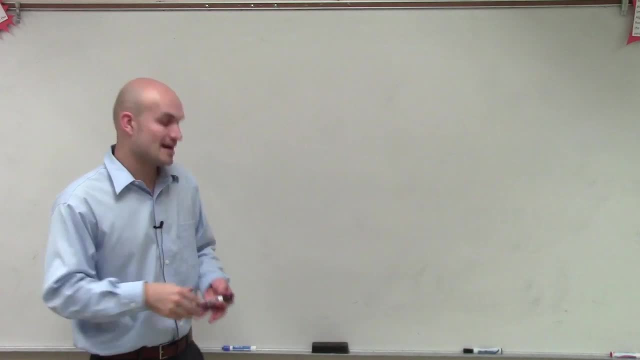 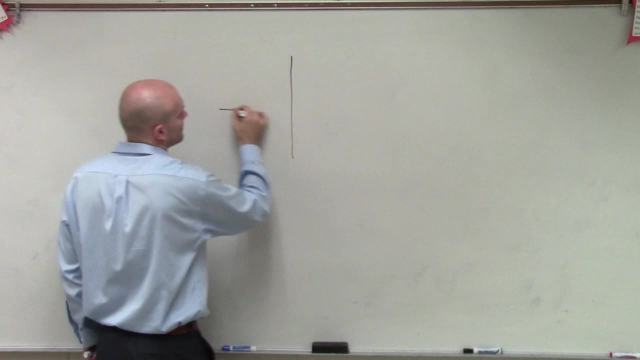 Now we're not going to get into how to find a line of symmetry. That's going to be a little bit further down in the course. But let's just kind of understand where exactly the line of symmetry is. So if we look at a parabola and let's just go with the standard equation, 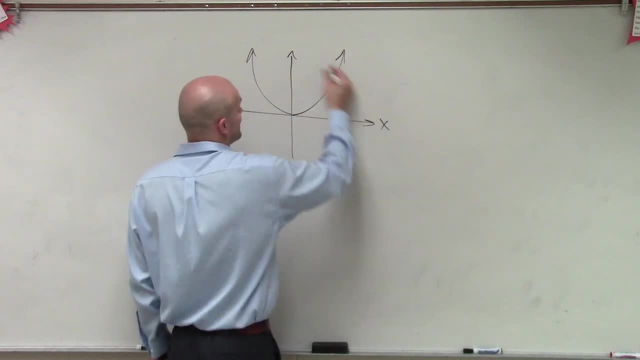 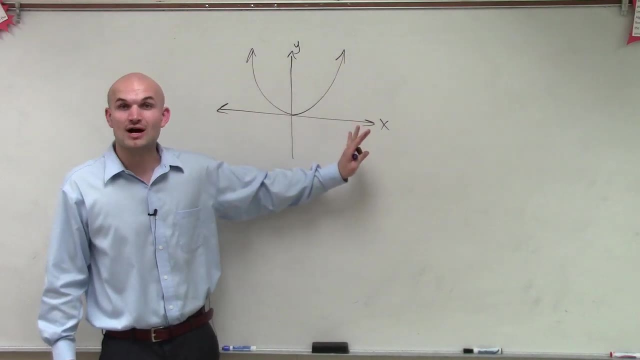 of a parabola. We're going to have our x-axis and our y-axis. What we notice is: is there a line that I could draw, where I could flip my line of symmetry? I can see that there's a line across the line and we're going to have the same graph. 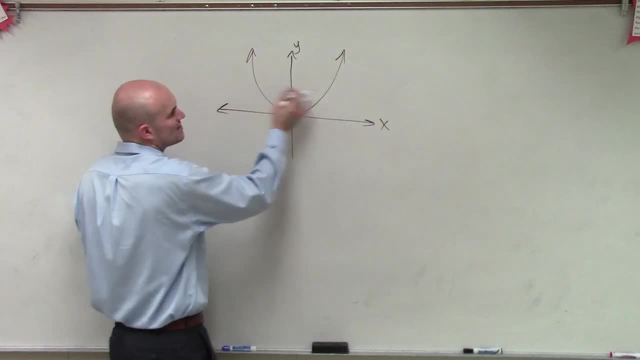 So, if you notice, I can't draw a line, a horizontal line, any horizontal line where I could flip it over the horizontal line, and it would be exactly the same. However, if I draw a vertical line, And in this case you can see that this vertical line is right on the y-axis. 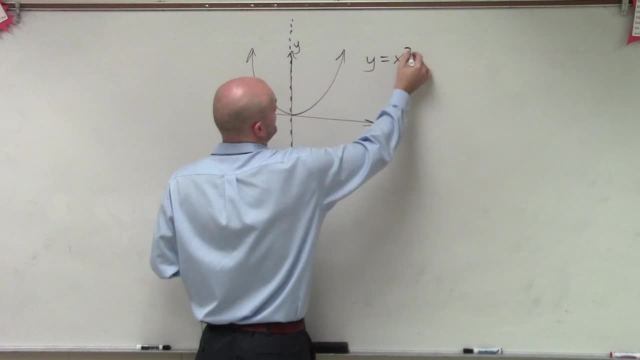 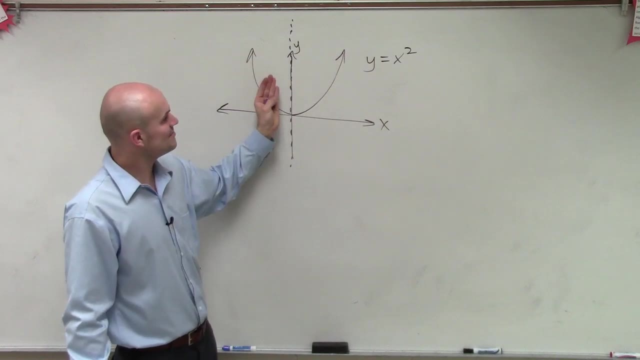 So when I have the parent graph, which for a quadratic is y equals x squared, the line of symmetry is directly down the middle, which is actually at the y-axis, And this is going is the line of symmetry, because I can reflect the graph. 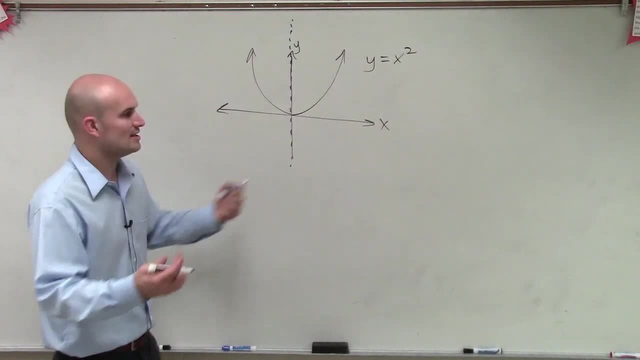 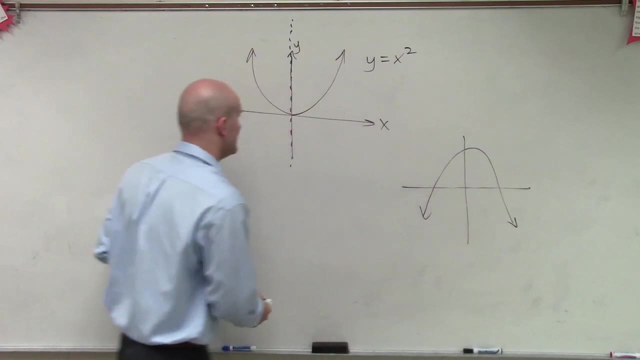 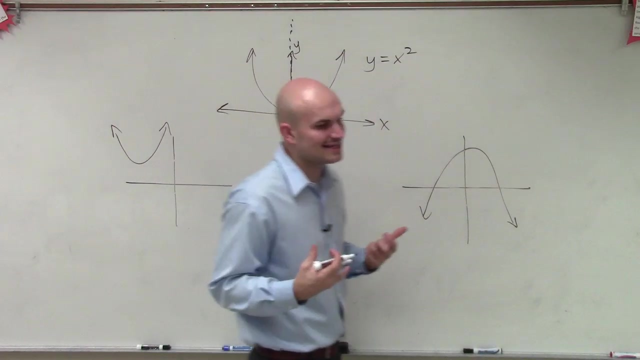 over this line of symmetry to produce the last graph. Now let's just go and take a look at a couple examples of parabolas, And they don't have to be on the origin, nor do they have to be opening upwards, And what I want to do is just show you where exactly. again, 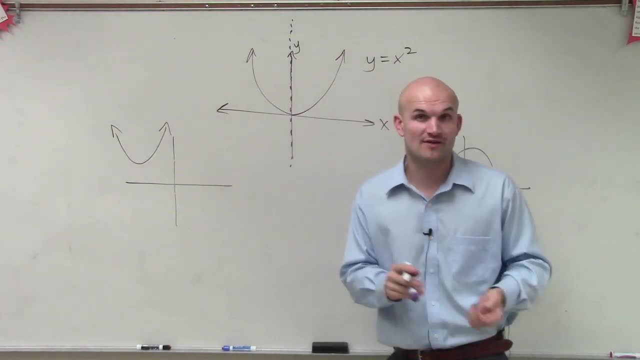 is our line of symmetry. Now there's a couple points that I'm going to get to. I don't want to get too far in advance with this, But what you notice is there's a minimum point here, And what we're going to talk about later. 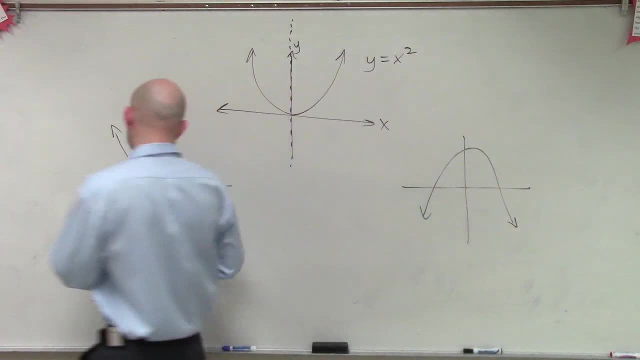 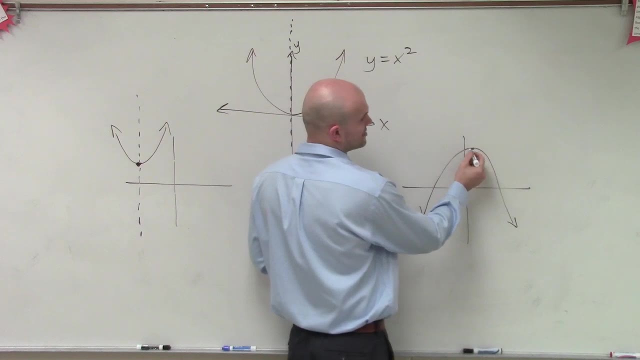 is at that minimum point, you can draw a vertical line which will create your line of symmetry. Over here you can kind of say, all right, here's my maximum point And through that maximum point is going to be my line of symmetry.